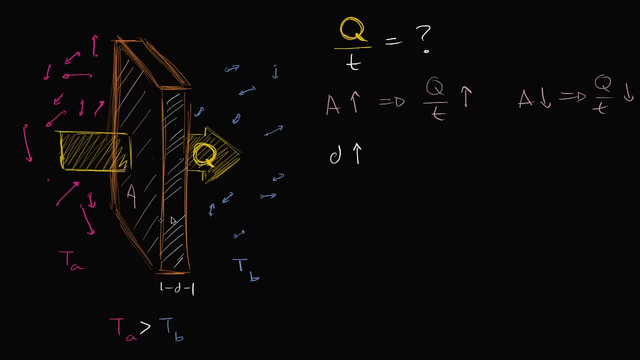 I would have more things that I would have to heat up to get it to a certain temperature, to before I can, or to which then can heat up the particles on the right, And obviously this is a continuous process. it'll always be happening. 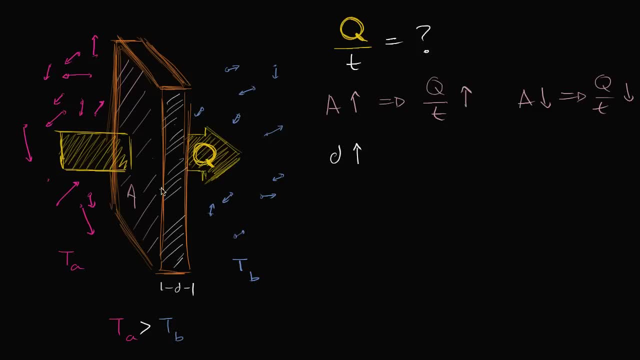 but there'll just be more stuff to heat up and it's going to take longer and more of that and more of that, more of that kinetic energy- that average kinetic energy- is going to get dissipated in this wall. So if this wall becomes thicker, 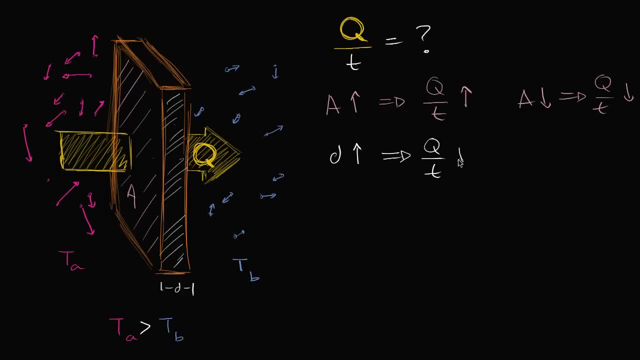 if the wall becomes thicker, then the rate of heat transfer is going to go down. Or, if you could, if the wall became thinner, if this depth decreased, then the rate of heat transfer, then the rate of heat transfer would go up. 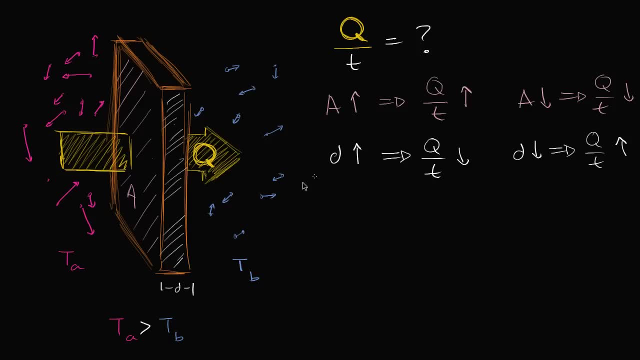 So you could say: the rate of heat transfer is going to be inversely proportional to the thickness of this wall. Now, what else could we think about? Well, we could think about the temperature differential. The temperature differential, that's T sub A minus. 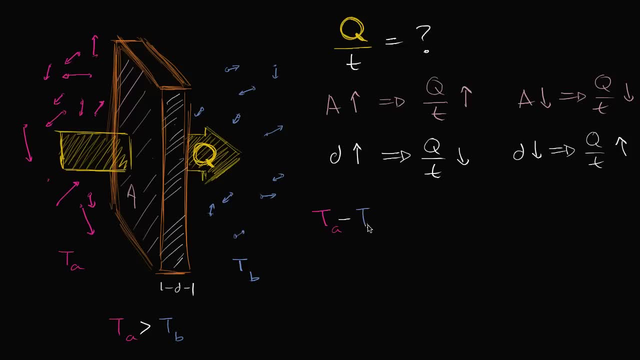 minus T sub B, Minus T sub A, Minus T sub B. Well, if this temperature differential, if this temperature differential were to go up, well, what's going to happen? Well, it's common sense that, well, if this is super hot. 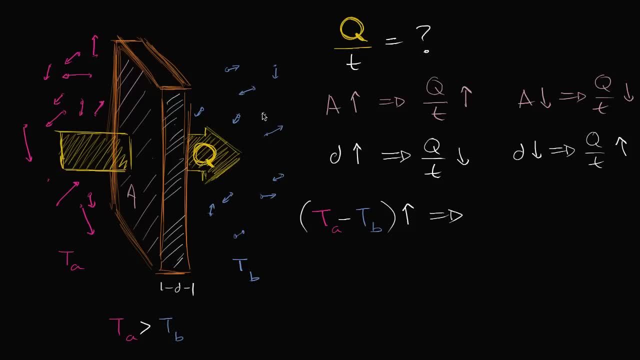 if this is super hot over here, this is way hotter than what we have on the right- well, we're going to have more heat transferred. So the rate of heat transfer- you're going to have more heat transferred per unit time- Your rate of heat transfer is going to go up. 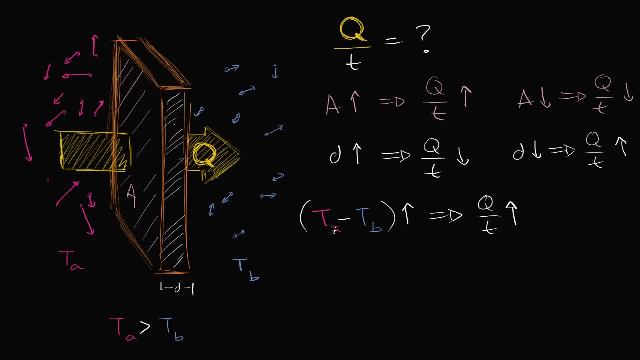 And likewise, if this differential were to go down, you could take the extreme case: if there was no differential, if T sub A was the same as T sub B, then you would have no net heat transfer, frankly, in any unit of time. 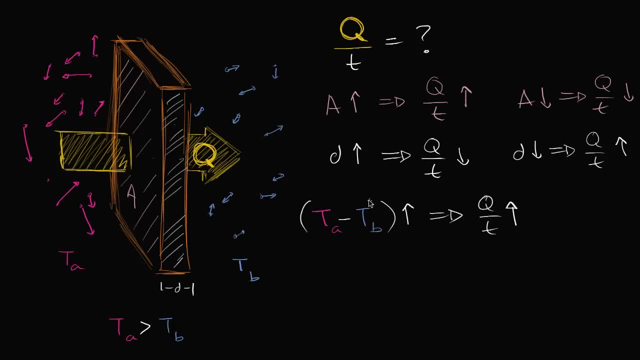 So it makes sense that the rate of heat transfer is going to be proportional to the temperature differential. So how can we encapsulate all of this intuition into, maybe, a formula for describing thermal conductivity, for thinking about how quickly, some how quickly- this heat will be transferred? 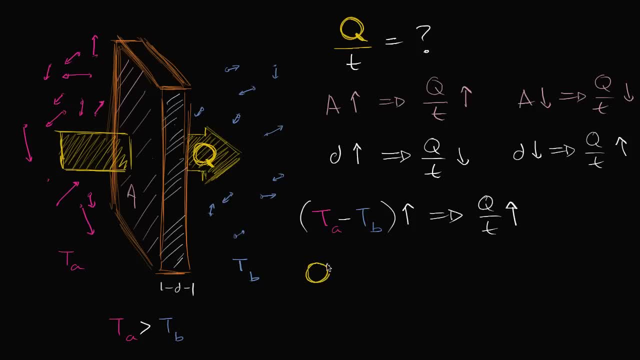 the rate of heat transfer. Well, we could say the rate, the rate of heat transfer, and this is really- hopefully it comes out of a little bit of common sense or an intuition of what would happen here- the rate of heat transfer. I could say it's going to be proportional to 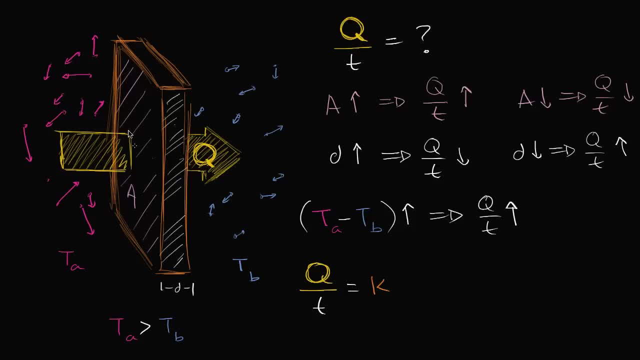 well, what are the things it's going to be proportional to? It's going to be proportional to the area. the more surface area we have on this wall, more contact area, the more heat we're going to have transferred per unit time. So it's going to be proportional to that contact area. 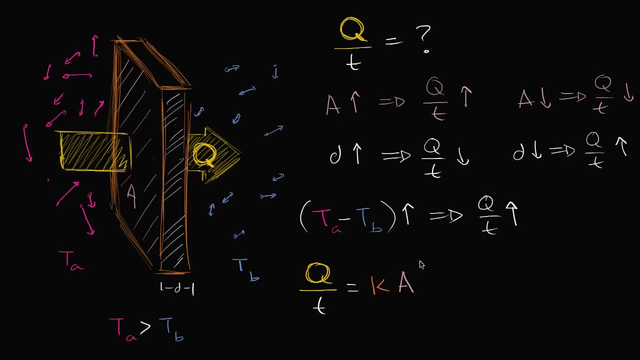 It's also going to be proportional to the temperature differential. So let's multiply this times the temperature differential, So T sub A minus T sub B minus T sub B, and it's inversely proportional to the thickness of the wall. So all of that over the thickness of the wall. 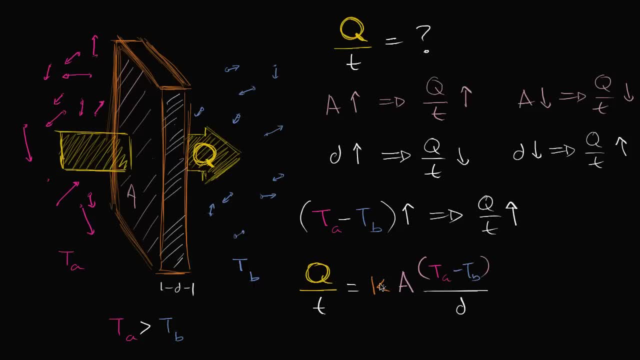 And now another thing that you might be saying: okay, I have this proportionality constant, but wouldn't this be different for different materials? For example, if this was a metal wall, wouldn't this conduct the heat quicker than if this was a wood wall? 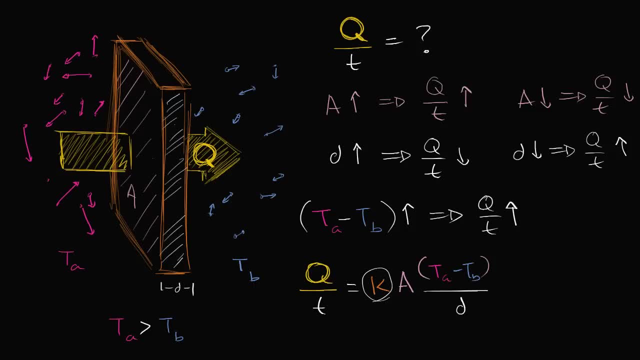 And you would be correct. This is a metal, wood, And so this K right over here. this is dependent on the material. So what is the wall made of? So material of the wall, And you can actually measure this thing, and different materials will have. 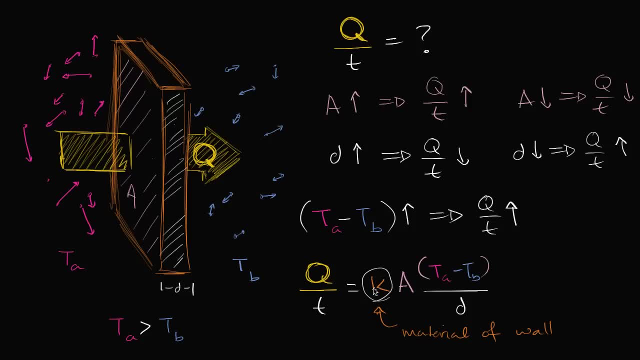 different thermal conductivities which this variable right over here would actually represent. So, going through a little bit of intuition, we were able to come up with what looks like a fancy formula, and you will sometimes see this formula a formula for thermal conductivity. 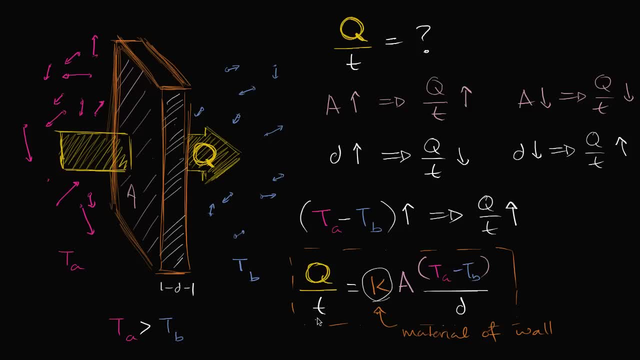 through a solid barrier, But it really comes out of, hopefully, common sense. The amount of heat transferred per time is going to be proportional to, and the proportionality constant is going to be dependent on, the material. Styrofoam, for example, would be very low here. 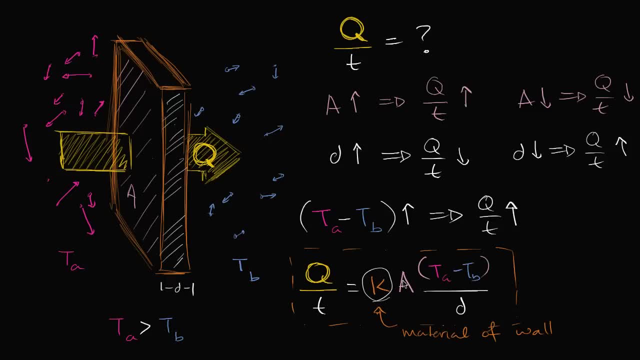 That's why coolers are made out of styrofoam, And it's going to be dependent on the area. It's going to be proportional to the area, the temperature differential and then inversely proportional to the thickness. So if you wanted to really insulate, 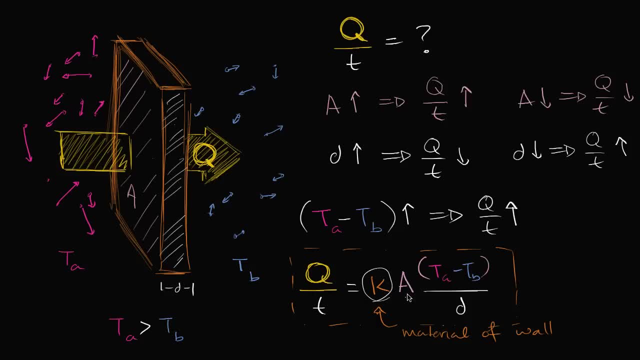 you would want to minimize surface area and you would want to maximize the thickness and you would want to have something with a very low thermal conductivity. So a thick styrofoam wall that's maybe shaped in a sphere might be a pretty good container. 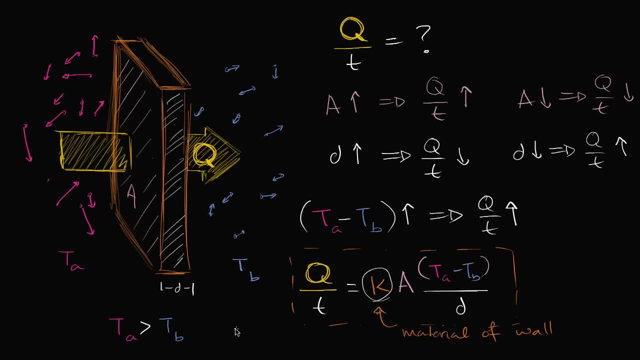 for keeping something hot or for keeping something cool.